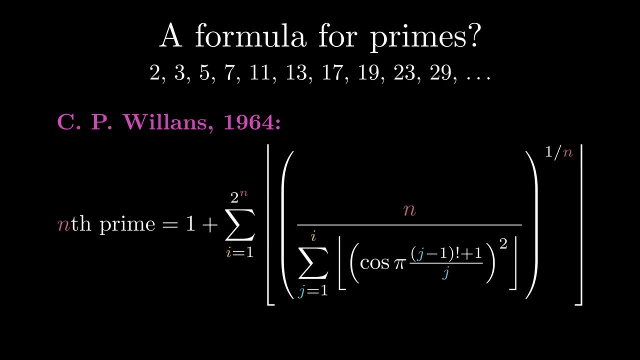 for it to digest you. Its components are all basic arithmetic and trigonometric functions, along with some ones twos and this pie sitting down here for some reason, And somehow this particular assemblage of functions that have nothing to do with primes on their own actually. 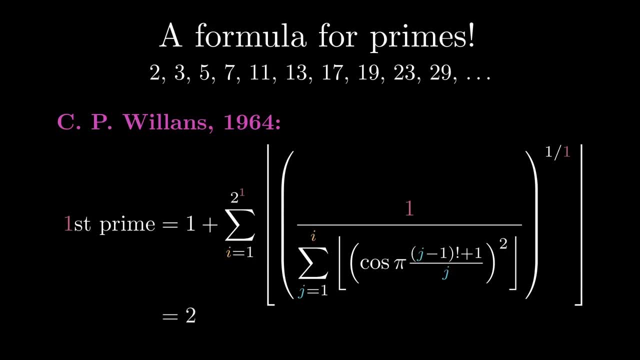 computes primes. Plug in 1, and it gives you the first prime. Plug in 4,, it gives you the fourth prime. Plug in 1000,, it gives you the 1000th prime. Amazing. So what kind of sorcery. 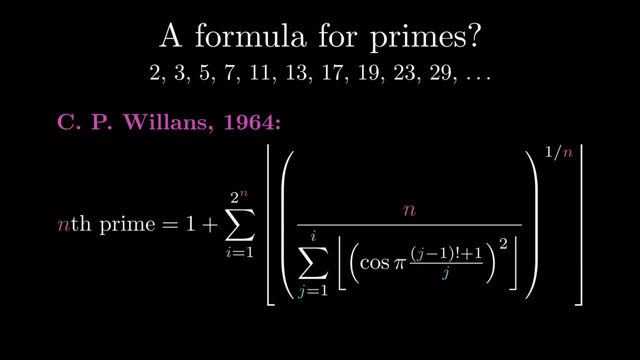 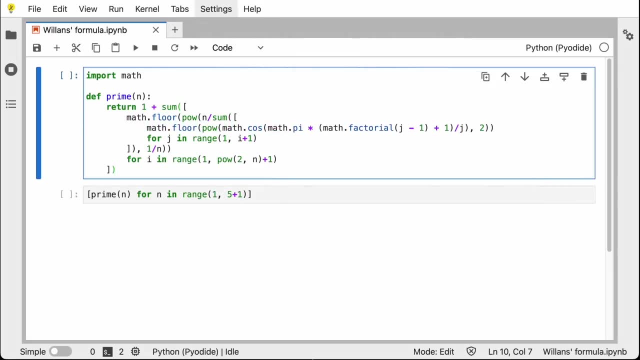 is this? Surely there's some trick, because the primes are supposed to be kind of randomly distributed among the integers, so there shouldn't be a formula for them. But on the other hand, if you type Willans' formula into your favorite programming language, it really does compute primes for you, at least for small. 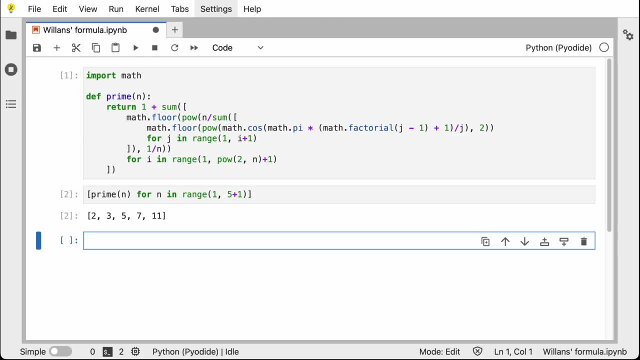 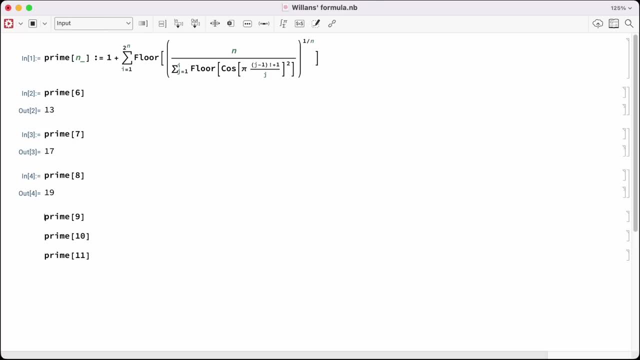 values of n before precision starts to become an issue. Symbolic software like Mathematica will give you primes for larger values of n. The thing is it's not particularly fast, And this is a hint about what the formula is doing and that maybe there are some caveats. 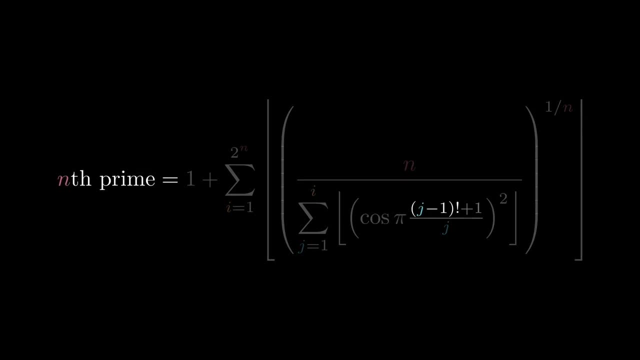 So let's see how it works, working our way from the inside out. The innermost piece is j minus 1, factorial. For example, when j is 5, this is 1 times 2 times 3 times 4, which is 24.. Then Willans tells us to add 1 and divide by j. When we 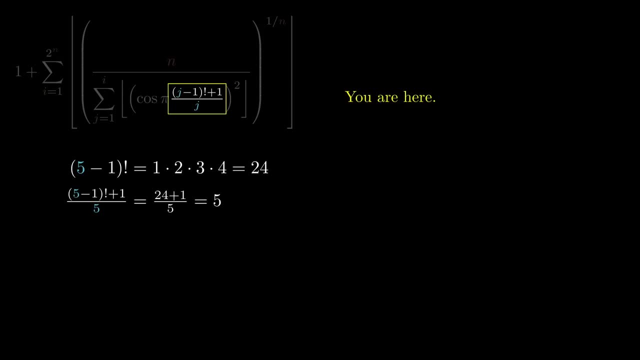 do this, for j equals 5, we get 5.. What if we change j to be 6?? 1 times 2 times 3 times 4 times 5 is 120.. Add 1 and divide by 6, and we get 121 over 6.. 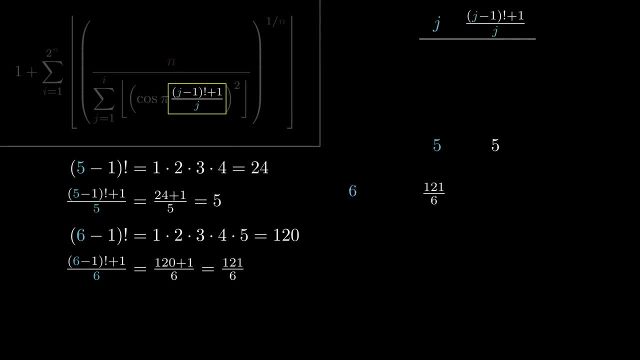 Here's a table with more values. Do you see a pattern? When j is a prime, it seems that we always get an integer. And when j is not a prime and not 1, then we don't get an integer. And this is the secret behind Willans' formula. 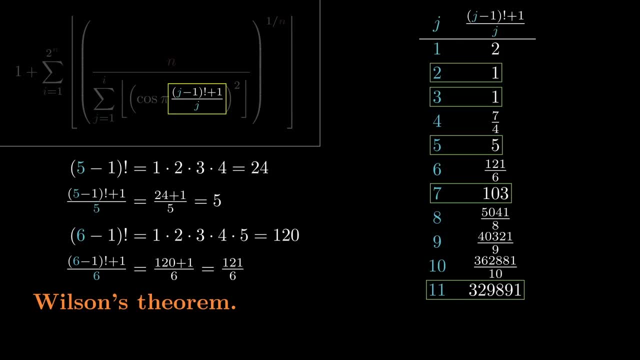 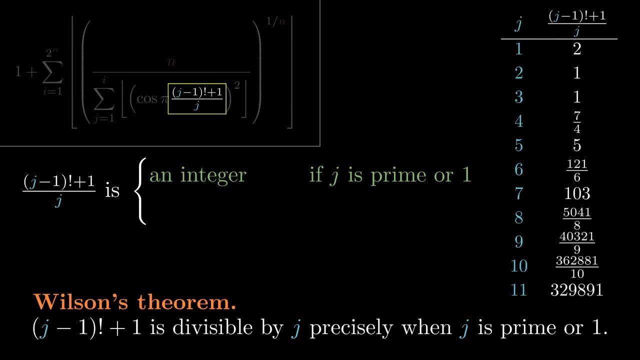 There's a theorem- called Wilson's theorem, not to be confused with Willans'- that says that 1 factorial plus 1 is divisible by j precisely when j is a prime number or j is 1.. This implies that when we divide by j, we get an integer when j is prime or 1, and a 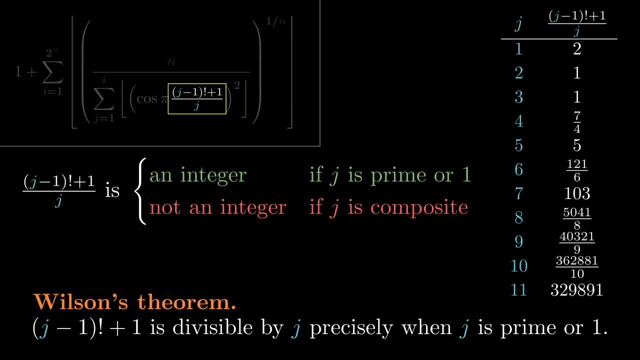 non-integer when j is composite. We've just built a detector for prime numbers, So how do we turn a prime detector into a prime computer? We can certainly use a prime detector to compute the nth prime in a not-very-clever way. 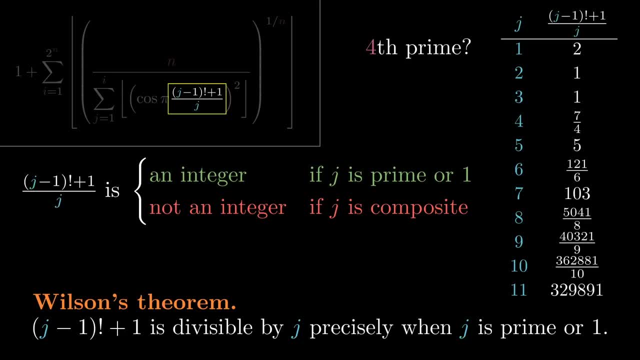 For example, to compute the 4th prime, we could start checking each positive integer for primality using our prime detector, Keep track of how many primes we've seen and stop once we've seen 4 primes Ready. 1 is not prime, even though our detector throws it in with the primes. so we have to be careful. 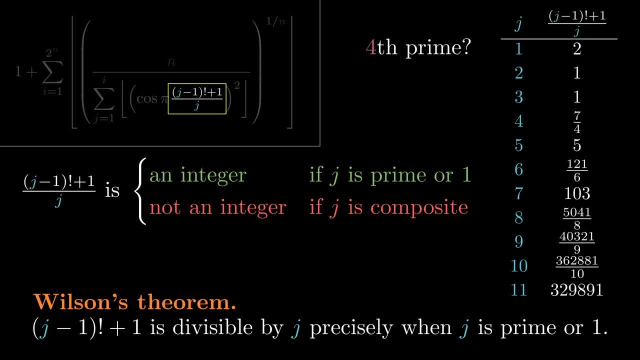 about that. But after 1, we're good to go. 2 is prime according to our detector, so it's the first prime. 3 is also prime according to our detector, so it's the second prime. 4 isn't prime according to our detector, so it's the second prime. 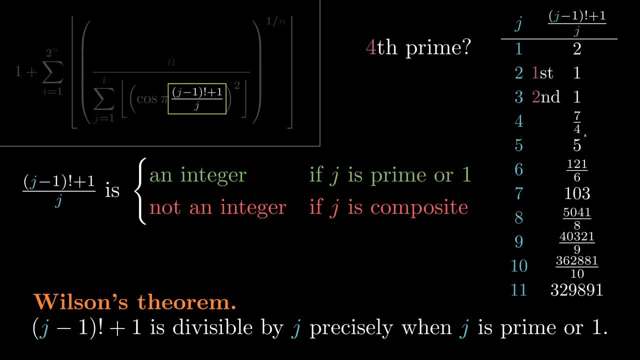 4 isn't prime according to our detector, so it's the second prime. 4 isn't prime according to our detector, so it's the second prime, But 5 is, so it's the third prime, and so on. What Willans does is implement this not-very-clever method in a very clever way. 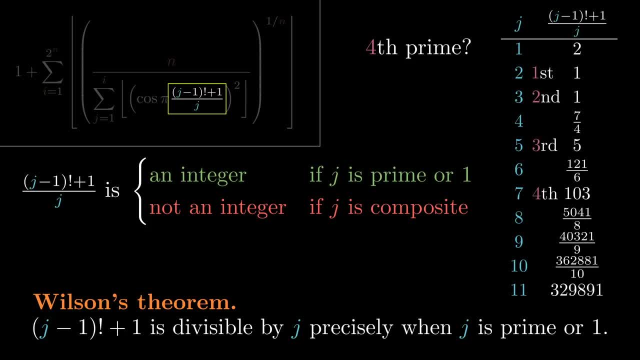 Because the thing is, if we were using a standard programming language, we could easily implement this with a while loop and a counter to keep track of how many primes we've seen. But what if we don't have a standard programming language at our disposal? 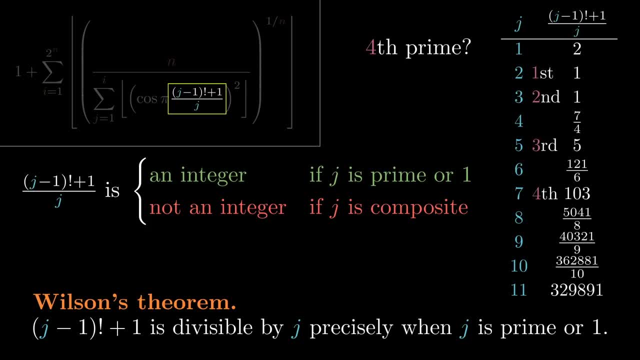 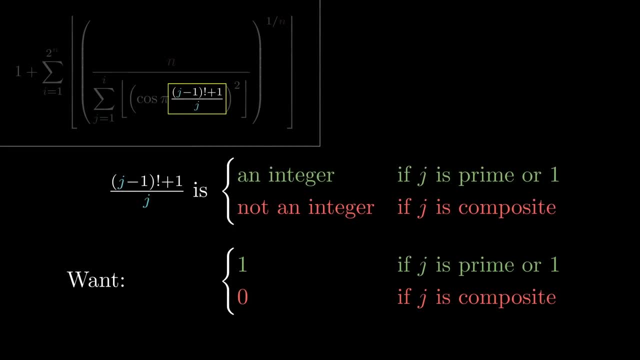 Well, Willans was still able to do it using traditional mathematical functions instead. First, it helps to modify our prime detector so that it outputs 1s and 0s rather than integers and non-integers. This will make it much easier to work with. 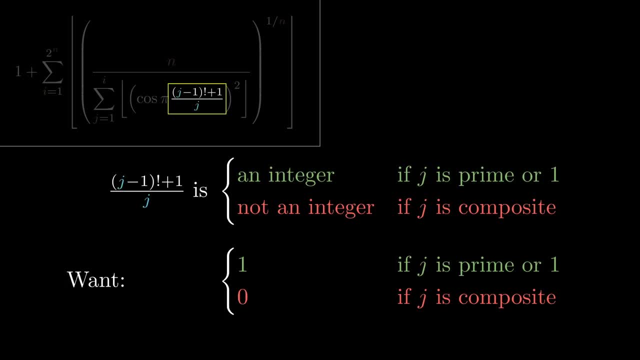 To convert integers to 1s and non-integers to 0s, we need an integer detector. So what kind of traditional function can distinguish between integers and non-integers? If we look back at the formula, we see what Willans came up with. 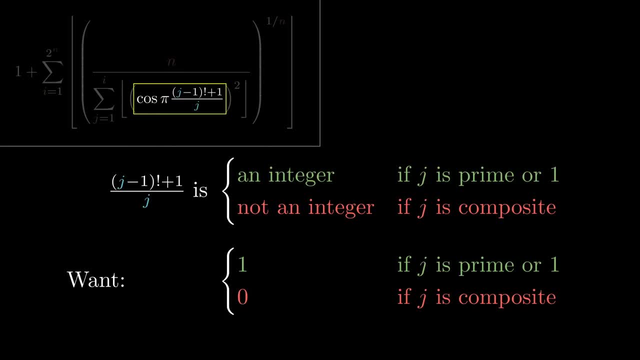 The next operation is to multiply by pi and plug the result into cosine. Let's see why this works. 1 is prime, This works. Here's a plot of cosine of pi x. It hits its maximum value of positive 1 at 0,, 2,, 4,, all the even integers. 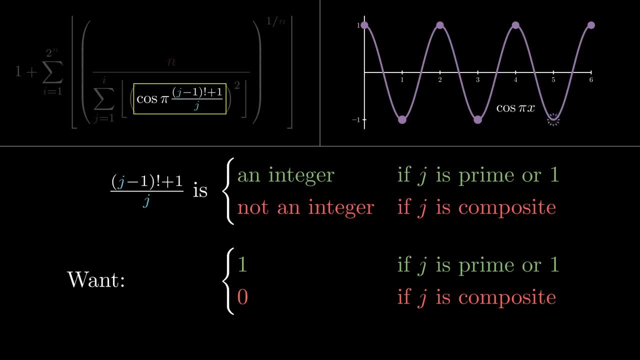 And it hits its minimum value of negative 1 at the odd integers. So when x is an integer cosine, pi x is either negative 1 or positive 1.. And when x is not an integer cosine, pi x is strictly between negative 1 and positive. 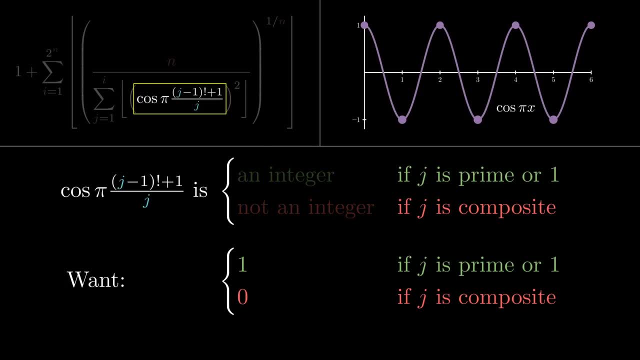 1.. This means that the cosine in Willans' formula is 0.. The cosine in Willans' formula spits out plus or minus 1 if j is 1 or prime, And it spits out a number strictly between negative 1 and positive 1 if j is composite. 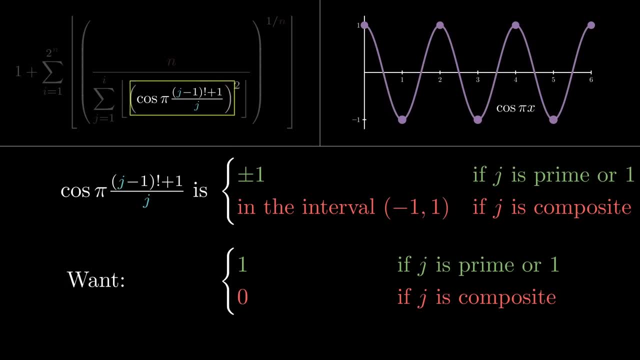 What's next Then? we square the cosine. The negative 1s become positive 1s when we do this. So the squared cosine in Willans' formula is 1 when j is prime or 1.. And it's a non-negative number that is strictly less than 1 when j is composite. 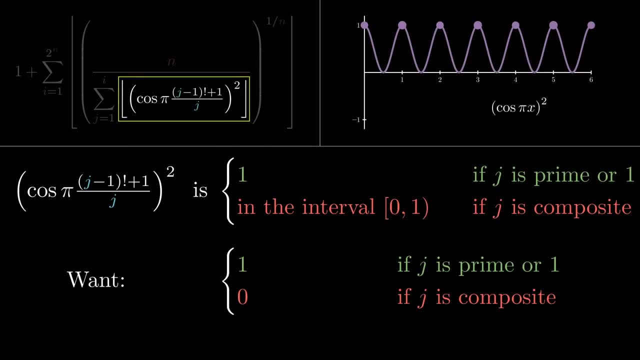 Then we take the floor. This leaves the 1s alone and collapses everything else to 0. So we get our improved prime detector that outputs 1s and 0s. It's 1 if j is prime or 1. And 0 if j is composite. 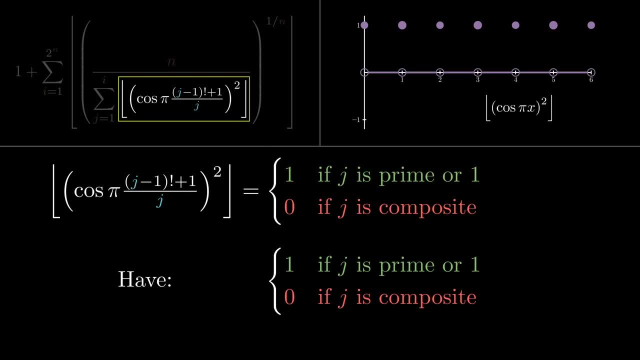 Isn't it beautiful that this is possible With this prime detector. we can start counting primes by summing over a range of values for j. For concreteness, here's the sum when i is 10.. j takes each value from 1 to 0.. 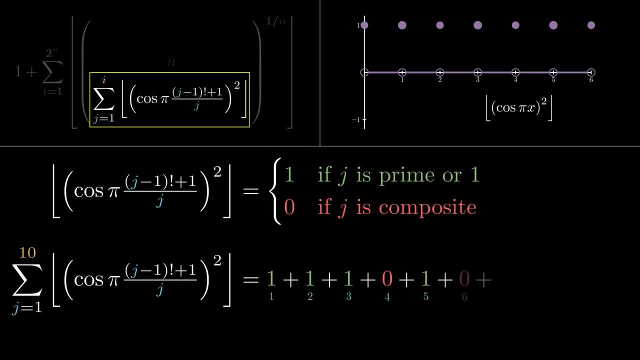 From 1 to 10.. And the detector contributes a 1 to the sum every time j is prime or 1.. There are 4 primes in this range, so the sum is 5.. In other words, this is the number of primes up through 10 plus 1.. 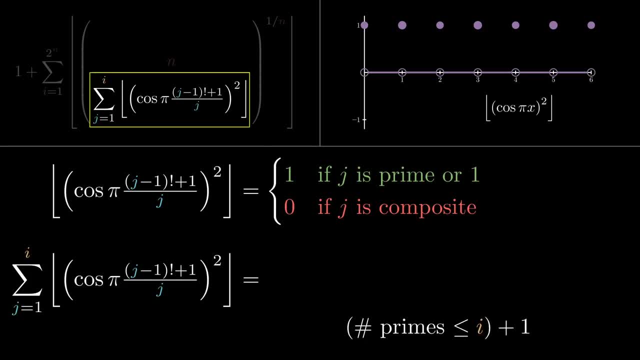 In general. if we sum up to i, we'll get the number of primes up through i plus 1.. So this whole complicated denominator has a very straightforward interpretation. It just counts primes. But wait, why are we counting primes? Willans formula is supposed to compute the nth prime. 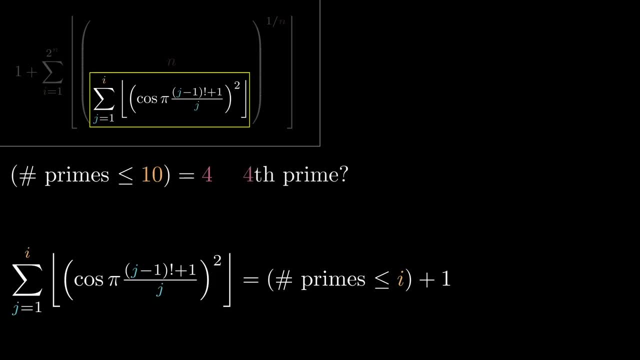 We just determined that there are 4 primes up through 10.. But we want to determine the 4th prime. Well, that's basically the inverse function of what we currently have. The idea is that if we want to know the 4th prime, then we ask: is the number of primes? 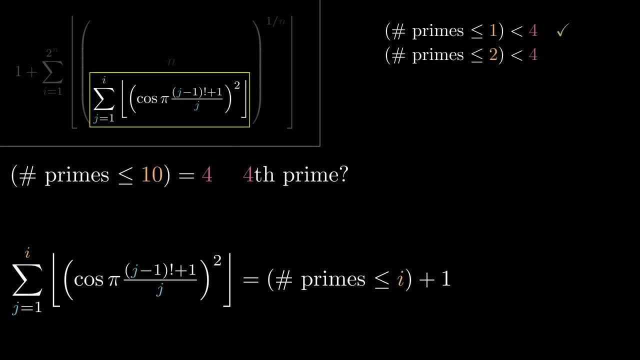 up through 1 less than 4?? Is the number of primes up through 2 less than 4?? Eventually the answer will be no, And the first time it's no will be when we're at the 4th prime. So the rest of Willans formula loops through. the question: is the number of primes up through? 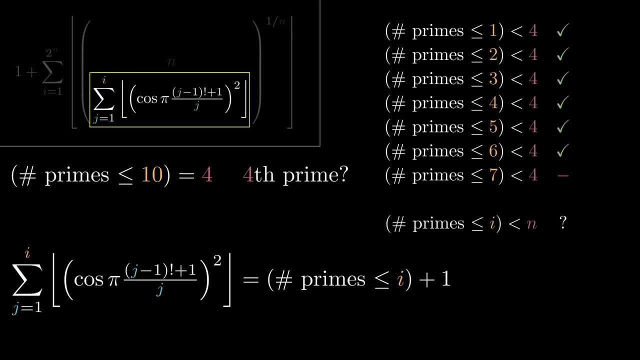 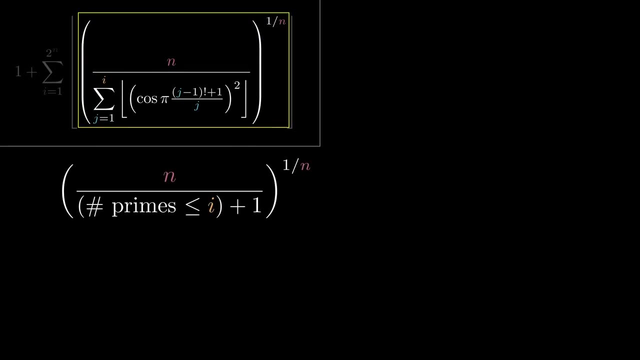 i less than n for various i, And this will tell us when we've reached the nth prime. It requires another bit of clever engineering, though. Let's look at the next component, where we finally see an n. It divides n by the number of primes up through i plus 1, and then raises the whole quotient. 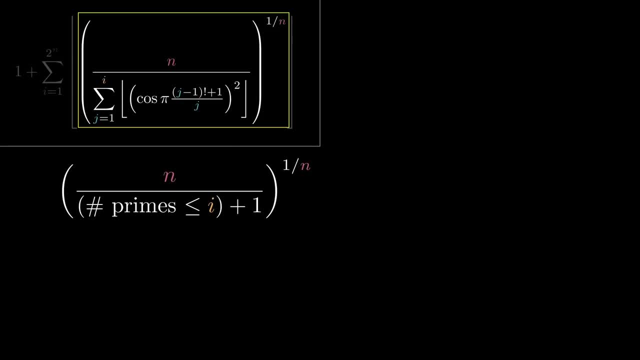 to the power 1 over n. When we evaluate Willans formula, we're going to be fixing n and varying i. but this part is actually easier to understand if we fix i and think of varying n. Take i to be 10 again. 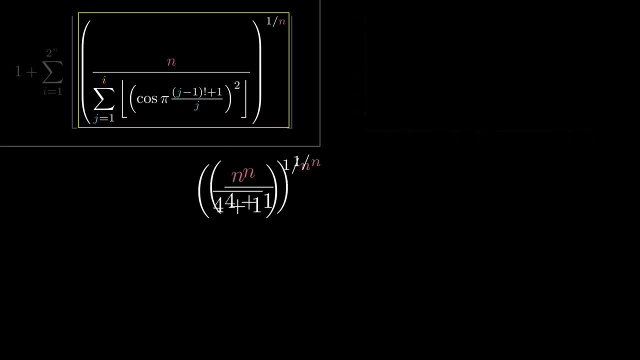 We know there are 4 primes up through 10.. Here is what the curve x over 4 plus 1 to the 1 over x looks like. We're going to take the floor of this function too, so let's see where it reaches height. 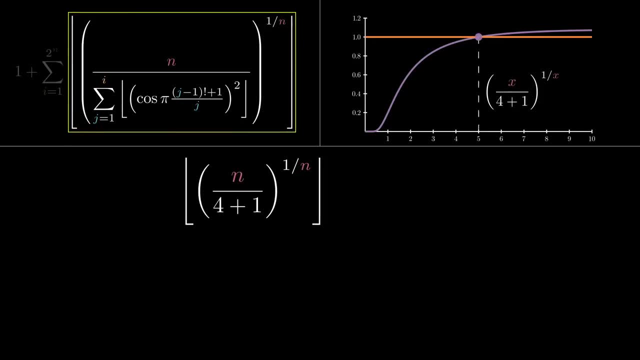 1.. Looks like it's at: x equals 5.. This makes sense because when x is 5, then the quotient is 1.. What happens to this curve for larger values of x? It looks like it might keep going up, but if we increase the range we see that it hits. 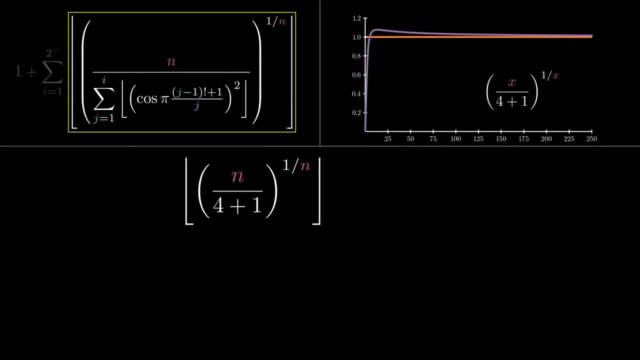 a maximum and then starts coming back down. That means that when we take the floor, we'll get 0 for integer values of x up through 4, and 1 for integer values of x greater than 4.. The result is that we've just implemented an inequality using nothing but arithmetic. 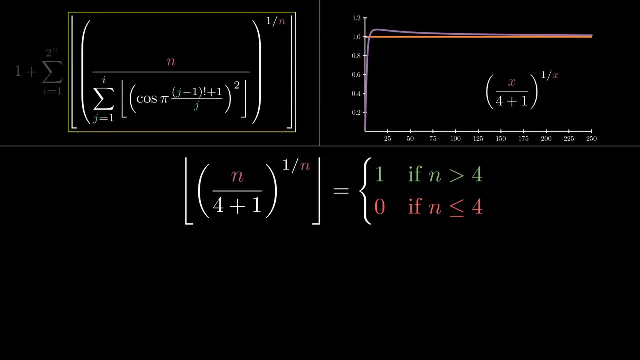 We have a detector for numbers that are greater than 4.. It takes some thought, but you can check for yourself that when you change this 4 to other values, this equation still holds In our current example. 4 is the number of primes up through 10.. 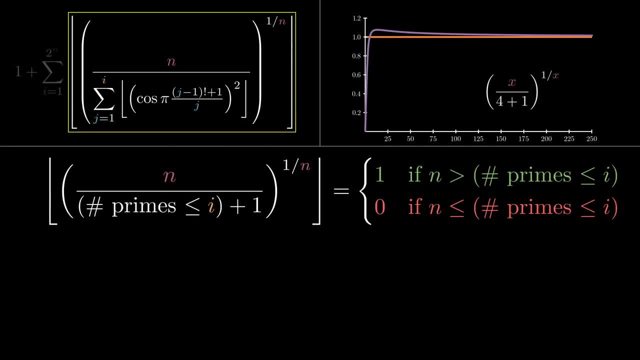 In general, this will be replaced by the number of primes up through i. This lets us answer the question: Is the number of primes up through 10?? Is the number of primes up through i less than n? Of course, when we go to use Willans' formula to compute the nth prime, it's not n, that. 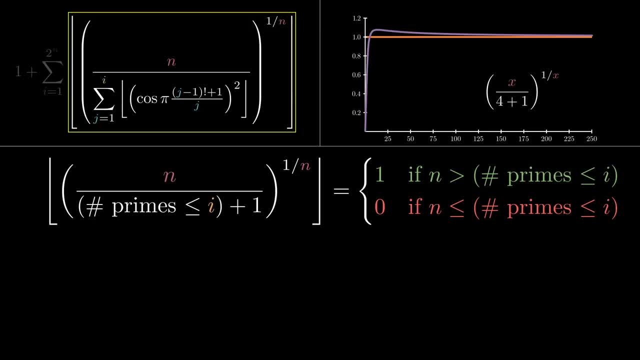 will change. It's i that will change because of the summation we're about to get to. So let's rewrite the conditions in this equation so they look more like conditions on i rather than n. The condition that n is greater than the number of primes less than or equal to i is equivalent. 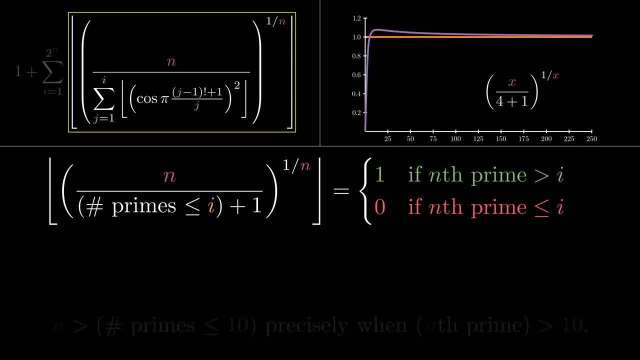 to the condition that the nth prime is greater than i. For example, n is greater than 4.. So we can write this equation: n is greater than 4, precisely when the nth prime is greater than 10.. Now reorder each inequality to put the focus on i. 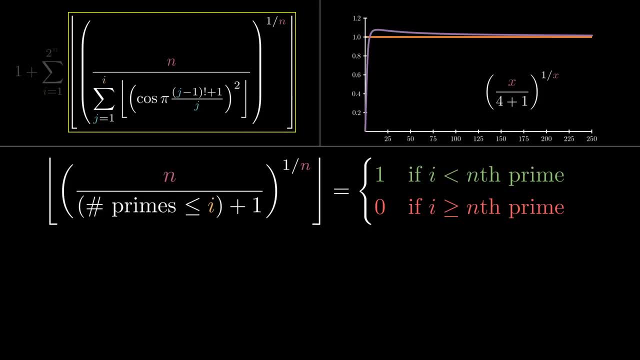 This is now a detector for numbers i that are less than the nth prime, And from here it's smooth sailing. The final step- well, almost final- is to sum over all i from 1 to 2 to the n. Again, let's look at an example. 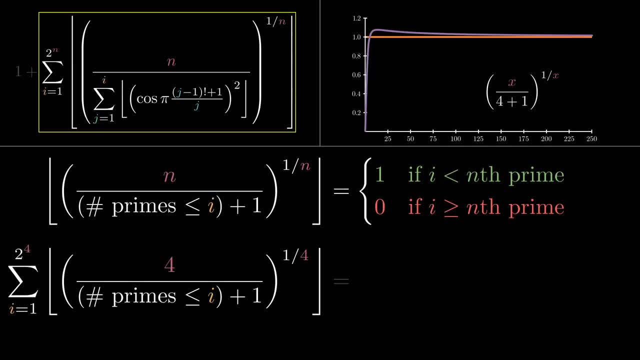 If n is 4, we're letting i go from 1 to 16.. For each value of i less than the 4th prime, we get a 1.. So overall we end up with 6,, which is 1 less than the 4th prime. 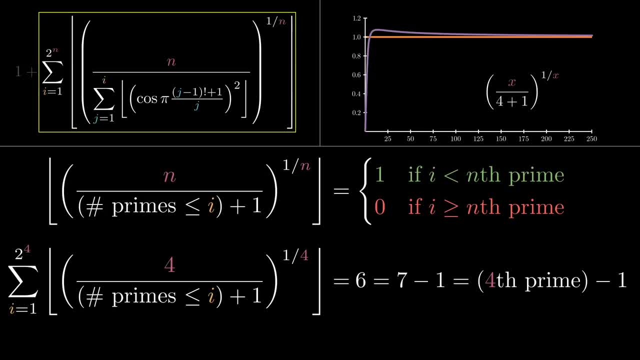 But why? is it enough to stop the sum at 16?? Well, we need to go high enough to guarantee that we go above the nth prime. Of course, we're trying to compute the nth prime, so we don't know exactly how high. 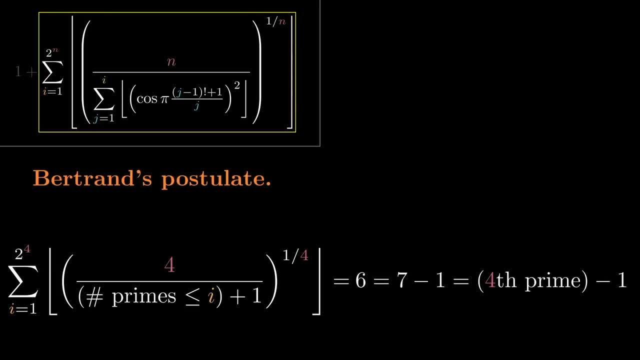 that is A very rough estimate, is provided by Bertrand's postulate, which was conjectured by Bertrand in 1845, and proved a few years later by Chebyshov. It says that for every integer m greater than or equal to 2, there exists a prime number. 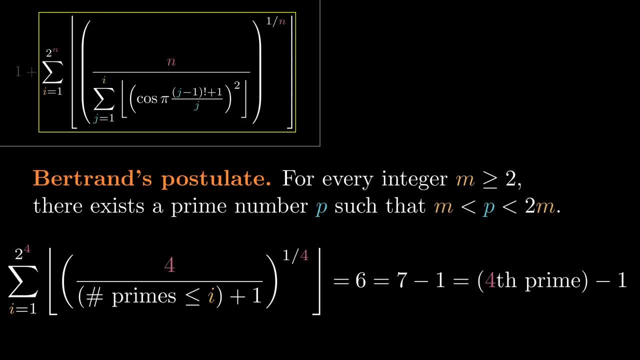 p between m and 2m. That means that there's a prime between 2 and 4, another prime between 4 and 8, another prime between 8 and 16, and so on … prime itself. Bertrand's postulate guarantees n primes between 1 and 2 to the n, So the 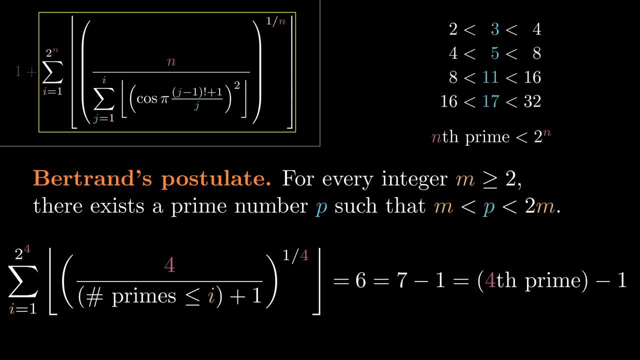 nth prime is somewhere less than 2 to the n. In reality the nth prime is far less than 2 to the n, but by now it's pretty clear that Willans wasn't overly concerned with efficiency. So the sum up to 2 to the n is guaranteed to include all values of i that 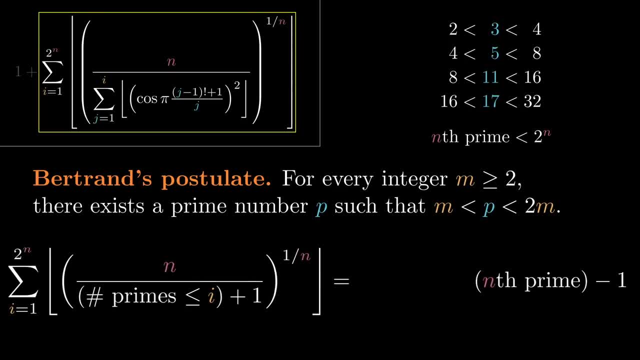 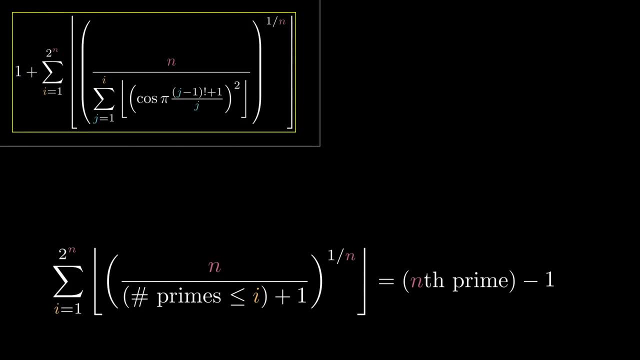 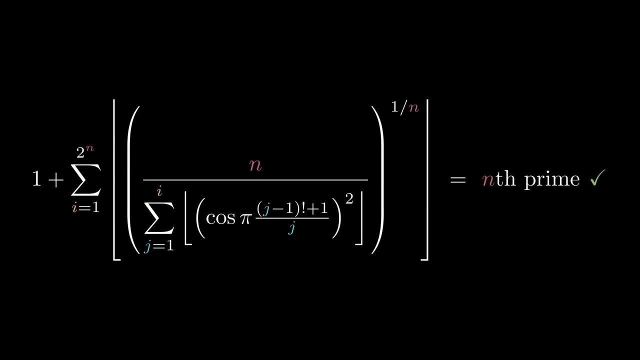 are less than the nth prime. Therefore, in general, this sum is 1 less than the nth prime. This is why the very last step is to add 1.. And there it is. We have a formula for the nth prime number, Or do we? 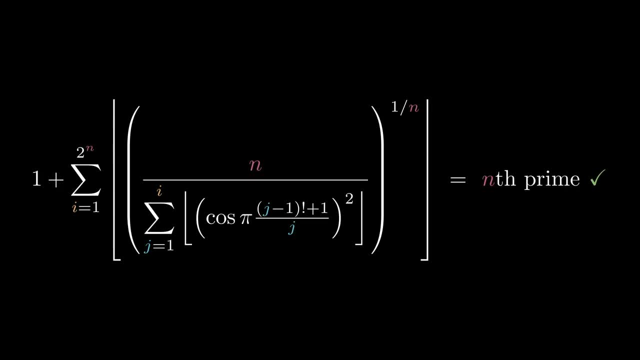 In practice Willans' formula is excruciatingly inefficient. We have a ridiculous sum up to 2 to the n. Evaluating each term in that sum requires another large sum and in that sum we have to compute j minus 1 factorial a bunch of times, which involves roughly j multiplications. 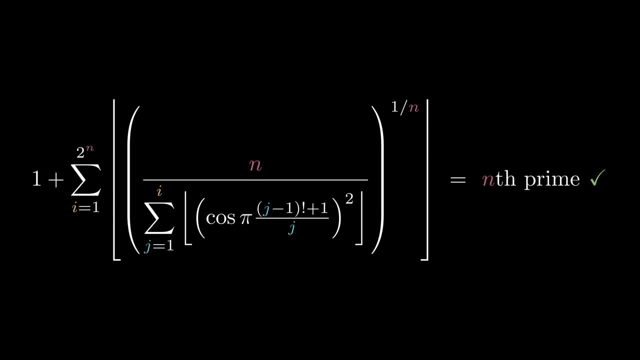 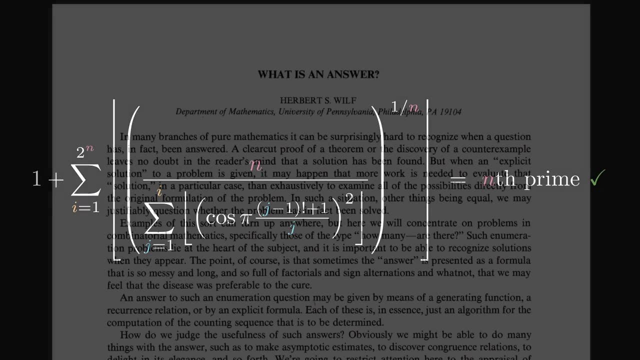 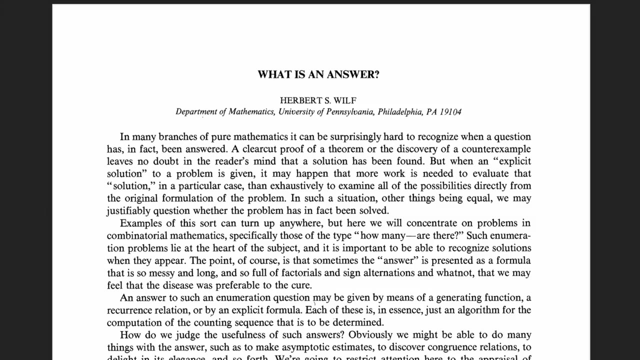 each. So even for reasonably small values of n, this formula takes forever. In 1982, 18 years after Willans' formula appeared, Herb Wilf, who has yet another name beginning w-i-l, wrote an article called What is an Answer, in which he argues that we: 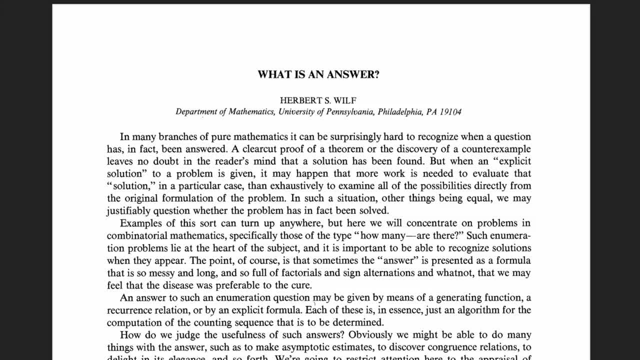 should judge a formula, like we judge an algorithm, by how quickly it produces results. We shouldn't accept an answer to a question that takes longer to compute results than the original definition of the thing it's supposed to be computing. He writes. The point, of course, is that sometimes the answer is presented as a formula. that is so. 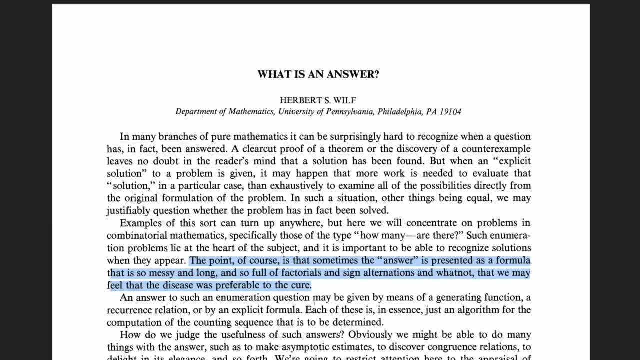 messy and long and so full of factorials and sign alternations and whatnot that we may feel the disease was preferable to the cure. Ouch Wilf doesn't mention Willans' formula specifically, but his description hits pretty close to home. 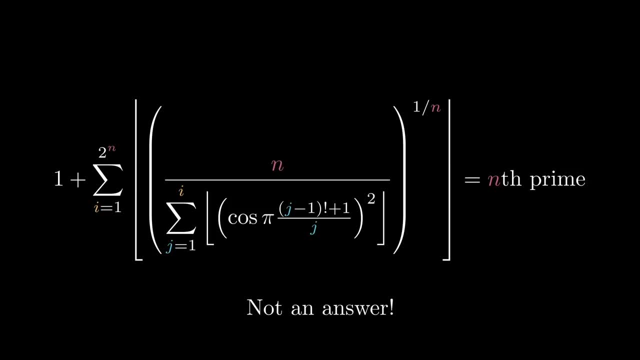 for Willans. Willans' formula definitely doesn't pass Wilf's test for being an answer to the question: what is the nth prime number, since there are faster and less complicated ways to compute the primes. So what's the point of Willans' formula? 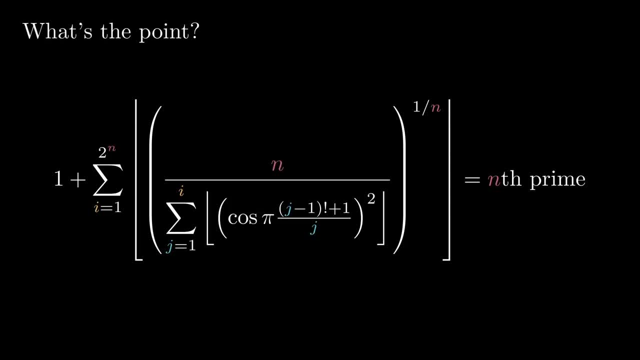 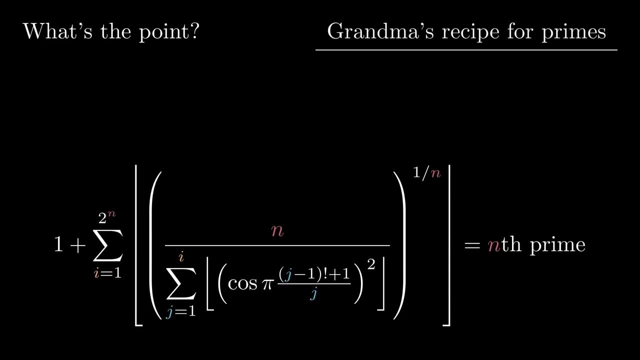 Well, you could think of it as a joke like: haha, here's a formula for the nth prime that is correct but totally useless. But there's something more interesting going on. At its core, Willans' formula isn't telling us how to compute primes, It's telling us what's possible to engineer with the.